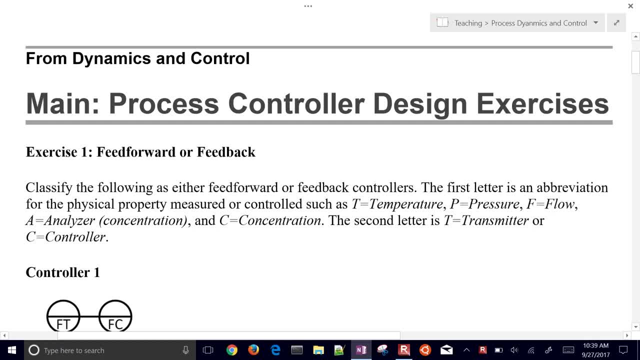 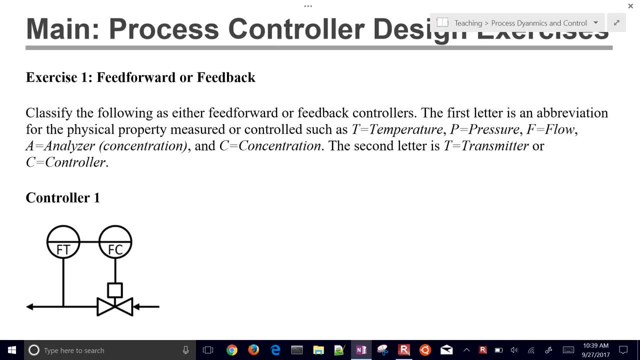 These exercises are to design process controllers or automation strategies. Let's go through this first exercise. We have a series of four exercises here. We're going to first of all classify feed forward or feedback control. So by looking at the system we'll know whether it's feed forward or 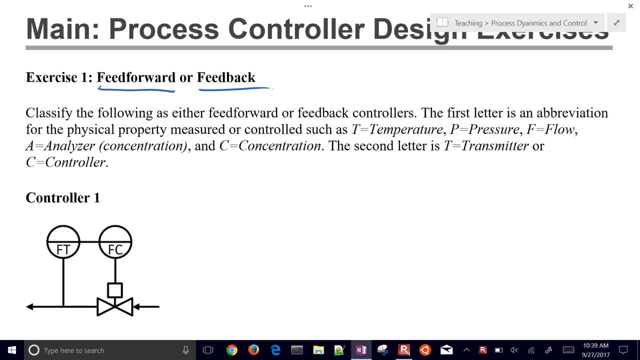 feedback. The main difference between the two is that with feedback, you're measuring and controlling the same thing. Your sensor is measuring the thing that you have a set point for and the two are the same quantity. So one thing that can give that away is whether you know it's a flow set point. 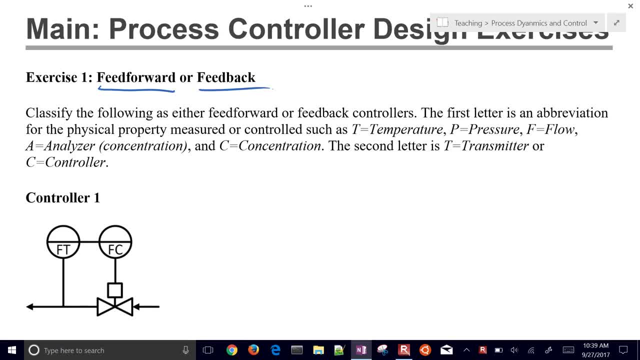 and then you're measuring that flow as well- Feed forward. you're actually measuring a disturbance of the system, So you're measuring a different quantity and trying to anticipate the effect that it'll have on the system. Now, in many systems you have feedback and then you add feed forward to. 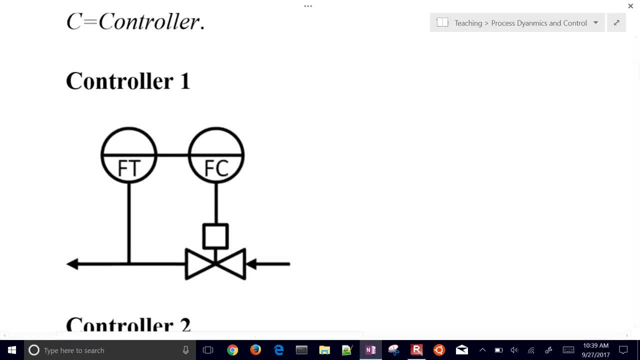 it. So let's go through these and just check them out and see if this is going to be a feedback or a feed forward control. We have flow coming through this pipe and we're measuring it at this point right here. Now the measurement is being sent to the flow controller and then the flow controller adjusts the valve. 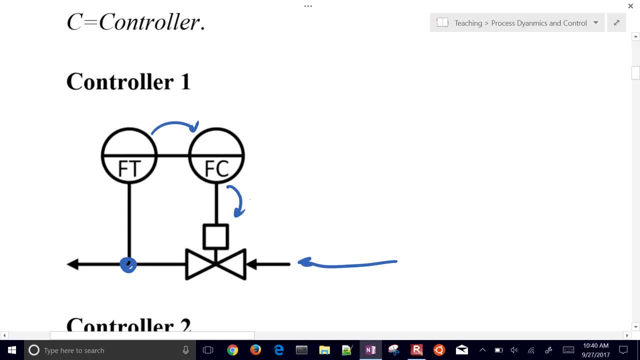 open or close to try to meet the new set point. In this case, the flow here, okay, is going to be the same as the flow here is going to be the same as the flow here, the same there. So we're actually measuring the flow, even though we're measuring it after the valve. It's going to be feedback. 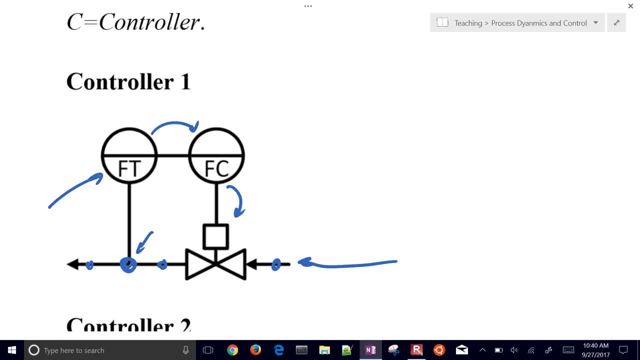 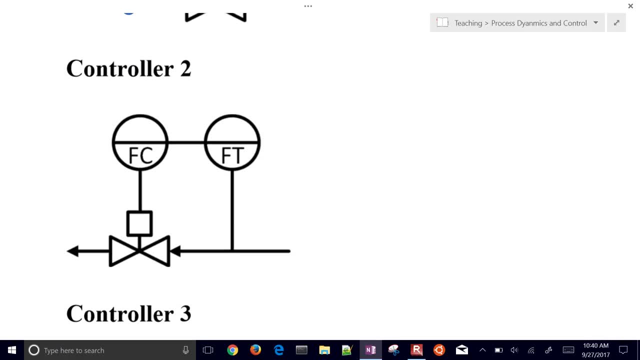 because we're measuring and controlling the flow and this is a feedback control system. Okay, number two, let's see if this is feedback or feed forward. So we're measuring the flow here and we're trying to control the flow. We have a set point of flow coming through this pipe. 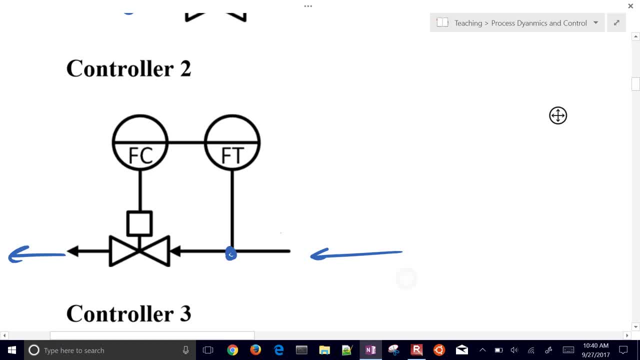 Now, if the valve is off the valve. it's going to be a feedback control system, So we're measuring the flow all the way. shut The flow is going to be zero here. it's going to be zero there If it's all the way. 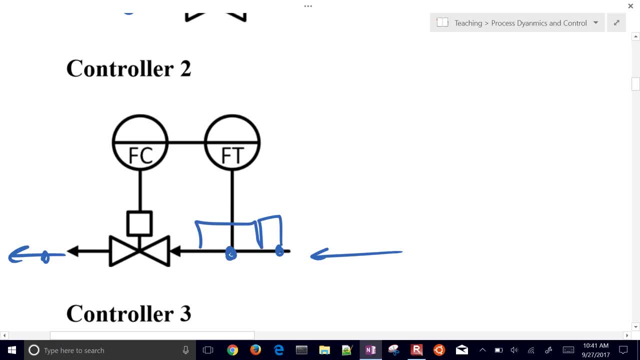 open. it's going to be the same at all of these places along there. Sometimes you could say: well, you know, if I close the valve and there's like a 10 mile stretch of compressible gas in there before I measure it, then you might have some delay in the measurement, but it's going to be. 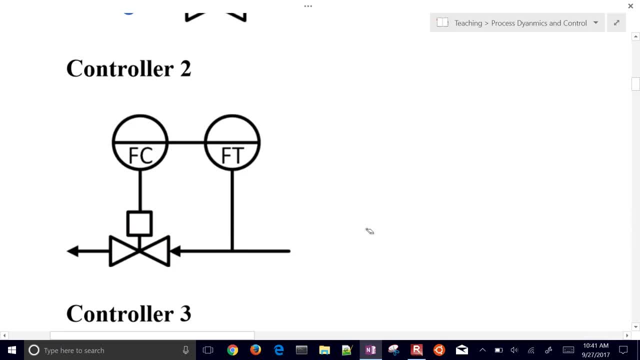 the same flow that you're measuring. Okay, so this one is actually going to be this one trips people up sometimes because they say, well, the flow is measured before we're actually adjusting it with the valve, so it must be feed forward. but it's not, It's feedback. 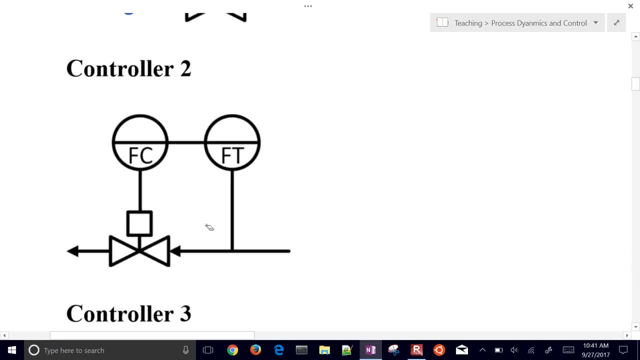 because the flow is the same everywhere in that pipe segment and we're measuring and controlling the same thing. Let's go on to this one. Here we're measuring the pressure at this point upstream of the valve, and so we're anticipating, let's say, a supply pressure changes. 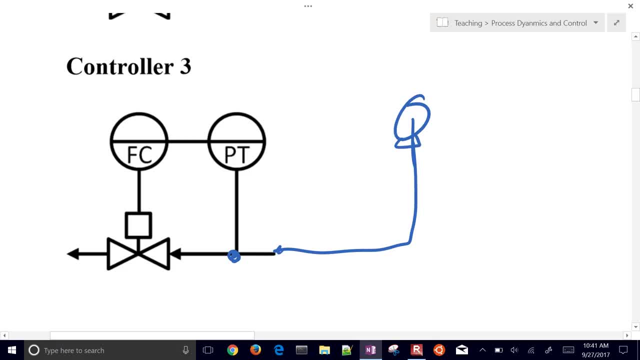 You know, we have maybe a pump that's supplying that, or you have other places that need this and so those are opening or shutting, kind of like when you're in your shower and somebody flushes the toilet, then sometimes it turns hot or cold, because you know mostly cold. well, I guess. 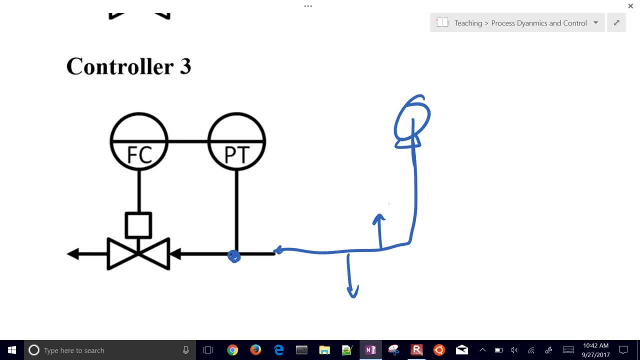 it would turn hot because somebody just reduced the pressure on the cold water line. Okay, and we're going to be measuring that upstream pressure and then proactively adjusting the valve opening in order to be able to compensate for that disturbance that affected the system. So in 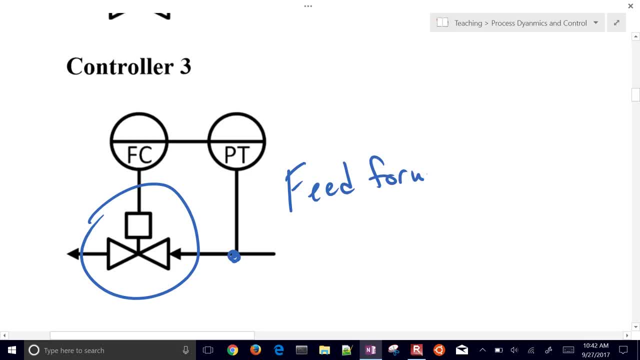 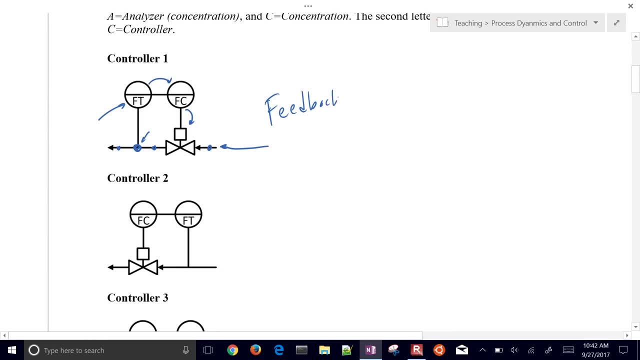 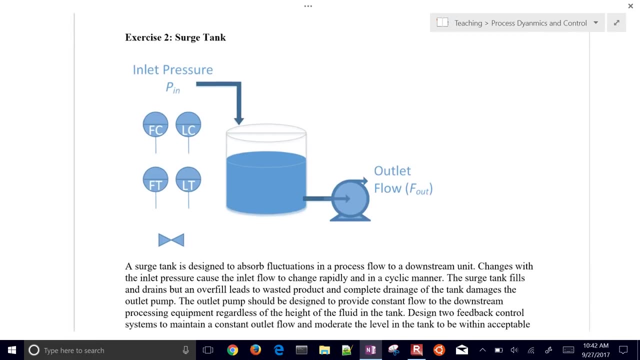 this case, this is going to be feed forward, and the other two are both feed back control. Okay, feed, two feedbacks and then one feed forward. Let's go on to the next problem. Here we have a surge tank and it's designed to absorb fluctuations in the process flow. so this: 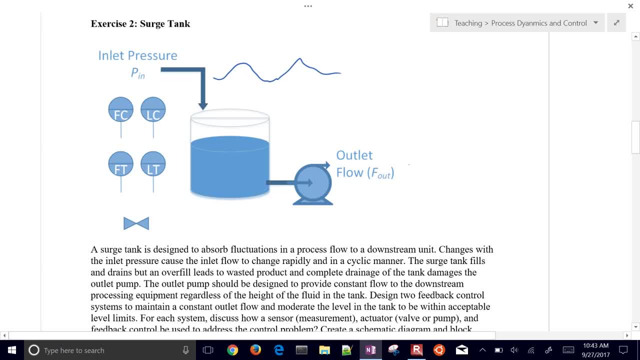 process flow could be going up or down, but we want to have kind of a consistent flow coming out of the system to some downstream units. So this is kind of like a surge tank that absorbs those fluctuations and and evens out the flow. Okay, so we have changes in this. inlet pressure cause this. 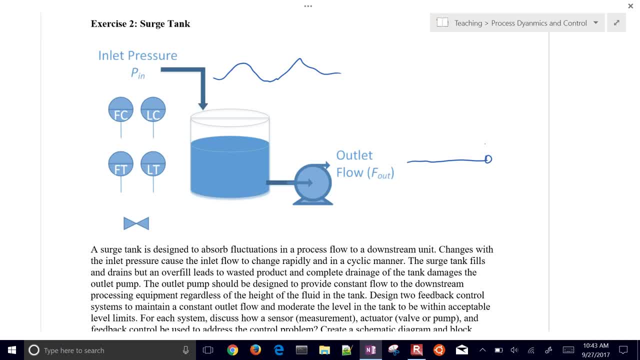 inlet flow to you know cycle, and we have all these elements right here. so we want to design a feedback control system. We have a valve, we have a flow transmitter, a level transmitter, a level controller and a flow controller. So we want to piece these together to try to design a system that's going to help us. 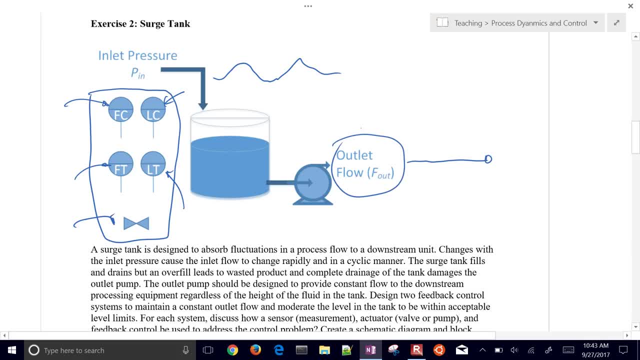 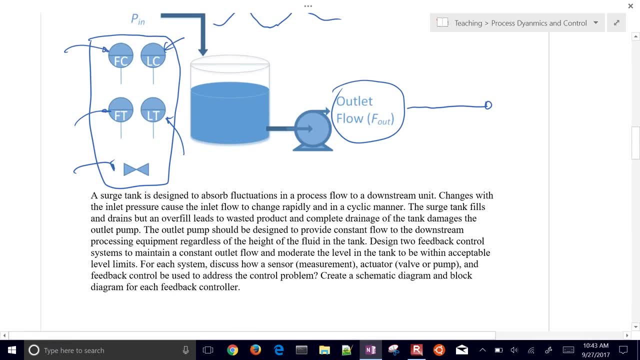 maintain this outlet flow right here, regardless of what the level in the tank is. So listen- and there's probably multiple ways it- you could do this: try to just maintain the level in the tank or you could measure the flow directly. so there is a couple different. 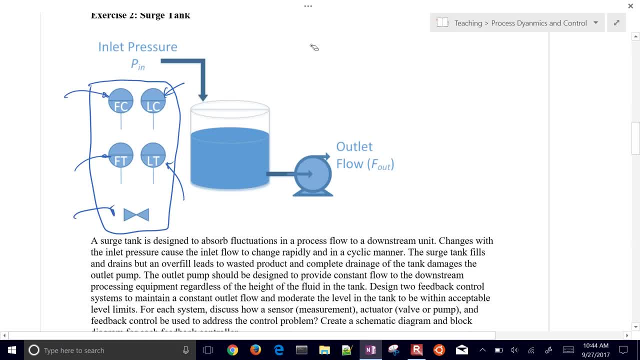 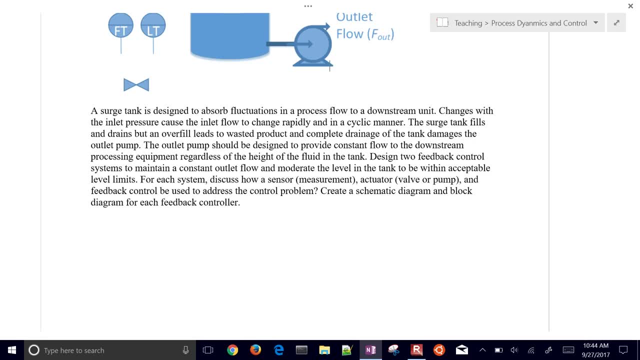 ways to think about this and also add feed forward elements to it as well. So let's look at exactly what we need to do for this. Ok, so for design, two feedback control systems to maintain a constant outlet flow and moderate the level in the tank to be within acceptable level limits. 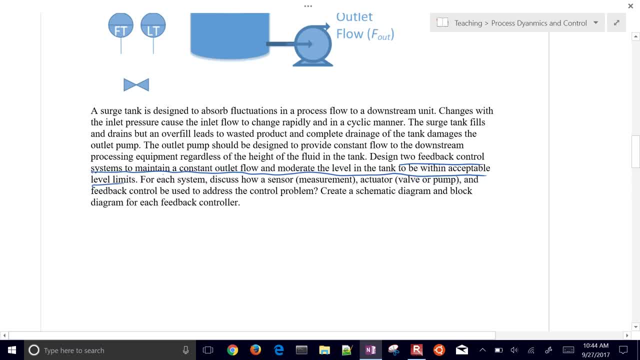 for each system. discuss how a sensor, actuator and feedback control can be used to address the control problem. create a schematic diagram and block diagram for each feedback controller. so let's come up with two different ones. maybe the first one is going to be just our flow controller. 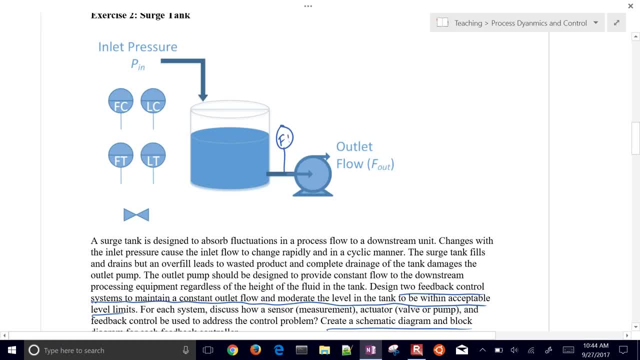 so we might have a flow transmitter right here and then this one might be: for example, we could add a valve right up here to the inlet, and then a flow controller is then going to adjust that valve. okay, so here's the very first one right here, and 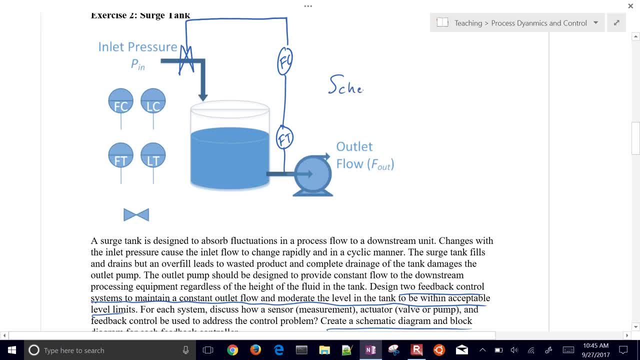 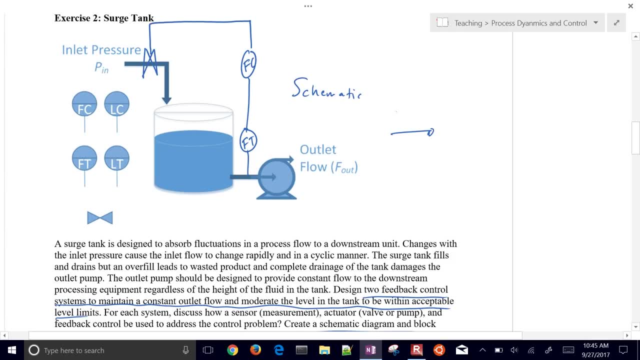 so let's there's. here's our schematic that we just drew, and then a block diagram where we have a set point. okay, this is going to be our flow set point coming out. we want to maintain a certain level. we're going to add a plus minus there and this is going to be. 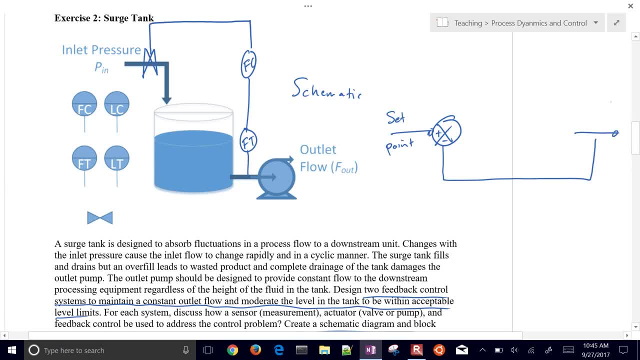 our sensor coming back. we're going to measure. uh, this is going to be our. i'll just write this in here. this is going to be our flow transmitter. it's going to be sensing what's happening with this flow. this is just a diagram of a flow of information. it doesn't necessarily represent a 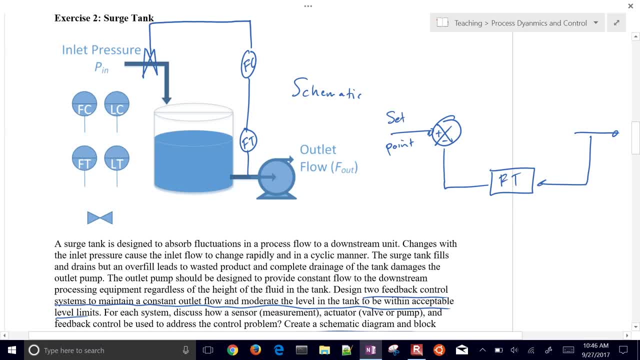 physical piece of equipment here and then we're going to be comparing these two. so this coming out is going to be the error, and the error is we often write that as set point minus pv and that is going to be the difference between the set point and the process variable. okay, coming from the 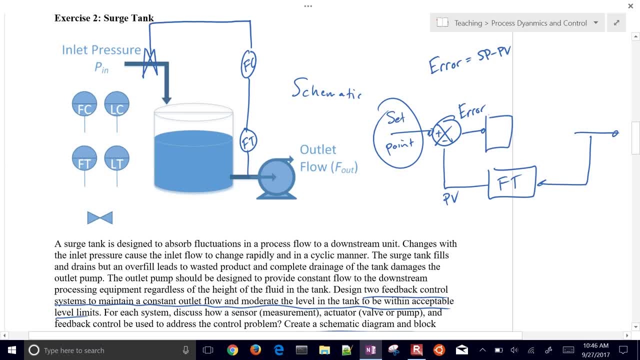 flow transmitter, then that's going to come into our controller- that might be something like a proportional integral derivative controller- which then goes to our valve and then that affects our process, you know, level and adjust the flow which is going to then inlet, which is then going to adjust the flow outlet. okay, so this is a model of like the whole. 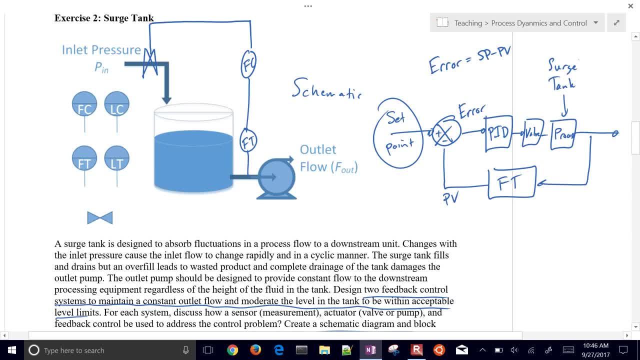 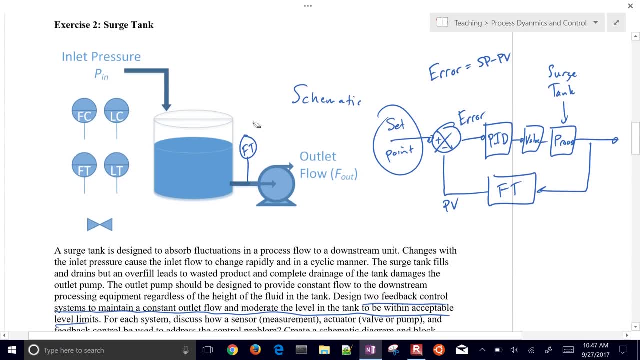 tank, the surge tank system. okay, there's our block diagram right there, so let's come up with just another one now. so we have, uh, there's our schematic. now let's see if we can use the levels. okay, this one's going to be a level transmitter, so if that level is, 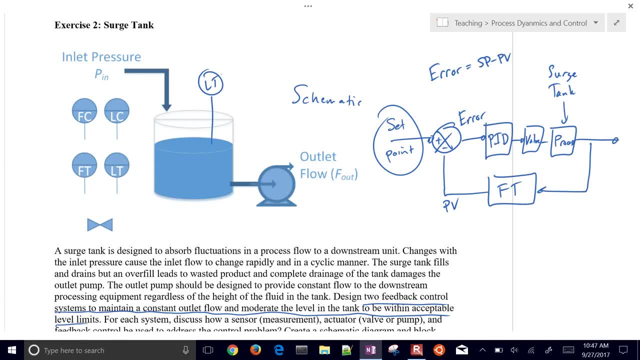 uh, too low or too high, it's adjusting, it's affecting the the flow coming out. so what we want to do is then then have a level controller. this is going to be a controller on the level and then that might be adjusting, for example, the flow coming in or out of. okay, from the upstream- okay. so here is a another. 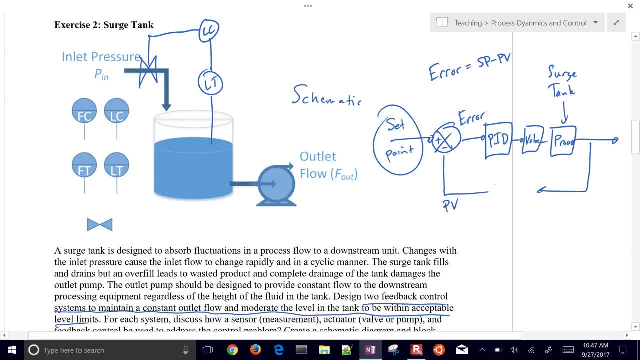 level controller. now, in this case, we just replace this flow transmitter with a um. this is going to be our sensor, right here. in this case, this is going to be our level transmitter. okay, the block diagram is essentially just going to stay the same. this is going to be our level controller. right here, our pid controller, and then we have a valve. 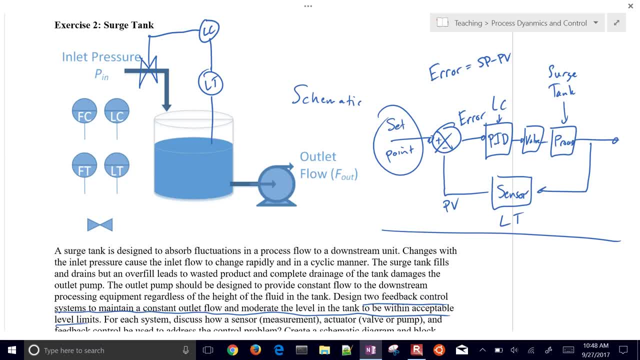 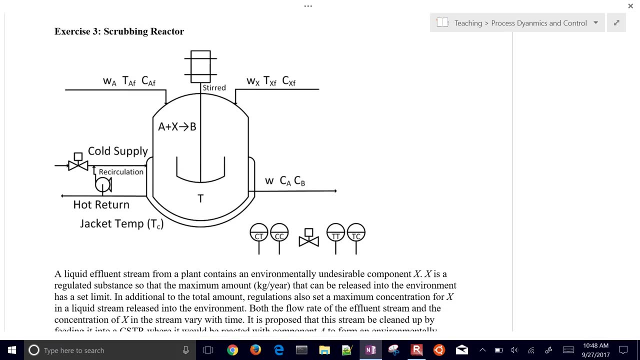 that then affects the process, so it just is really changing which quantity we're measuring, and then the controller then sends that signal again to the valve, okay, so, uh, let's go on to the next one now. so we have a more complicated system. this is a scrubbing reactor, where we have 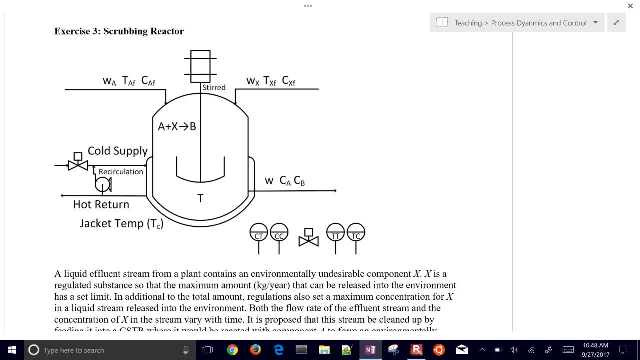 this reaction of a plus x goes to b and this liquid effluent is coming out. it needs to be cleaned up before it goes, let's say, into a lake. okay, let me draw a duck swimming. so you know that's a lake and we want to keep that clean. so the fish. 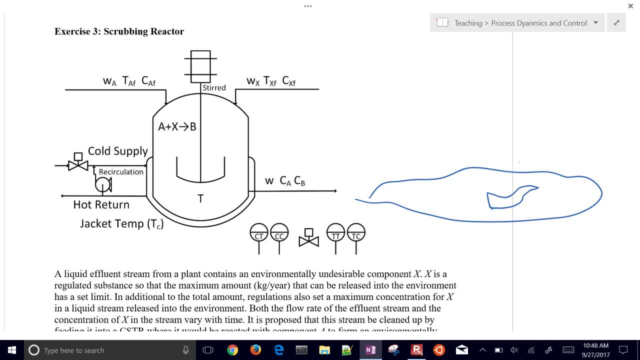 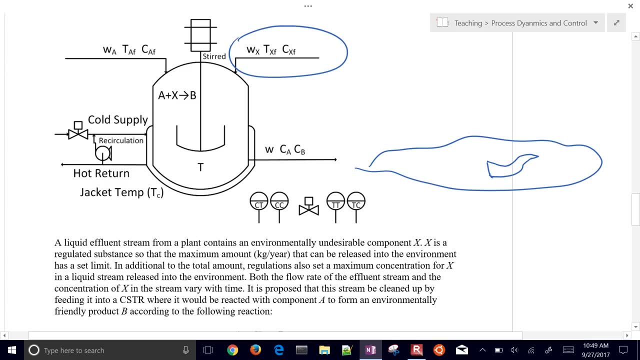 and the ducks and all the other plants stay healthy in that lake. and we have this component x right here and that helps us clean up our, our waste and but it's it's very expensive, so we don't want to use. we want to use the right amount of it to just be able to clean up the waste, but not. 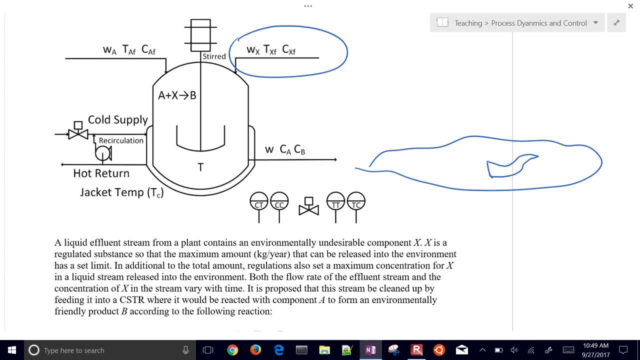 dump excess of that cleaning agent into the lake either. okay, so, um, oh, you know what i messed that up? component a is the one that, uh, is the expensive one. okay, let me back up there. this is the one that was going to be our cleaning agent. okay, and this is our effluent that we want to get rid of again. here's the lake i want to get rid of. 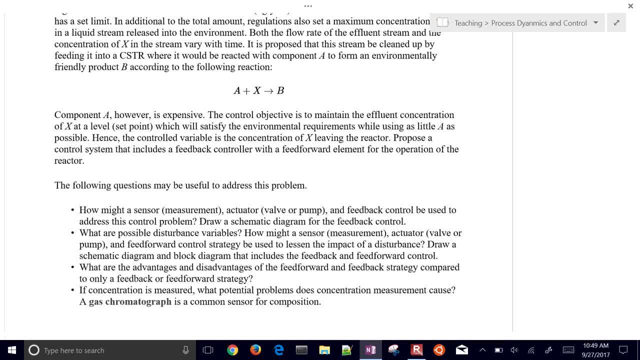 that, and then we can, you know, get rid of the other components so we don't have to go over that. so let's- uh, let's- design a feedback control system that's going to be able to help us regulate this outlet concentration we have. we want to propose a control system that includes. 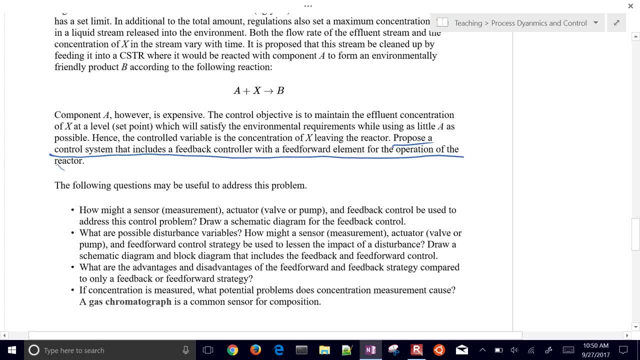 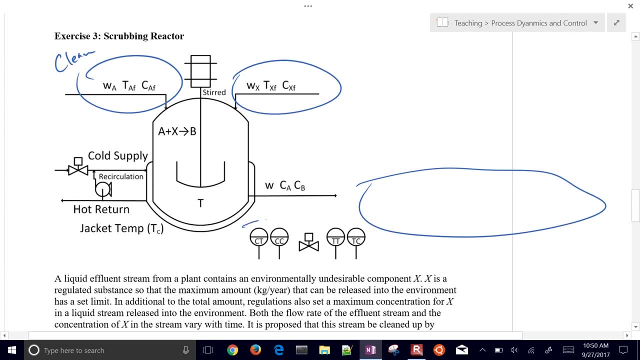 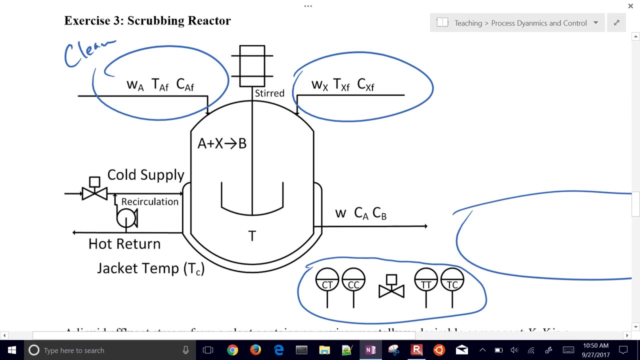 a feedback controller with a feed forward element for the operation of the reactor. so it's very important we don't go above a a certain limit, okay and so? so let's, we have this equipment right here that we can use to help us design this feedback controller. so what we might do then is: then we know. 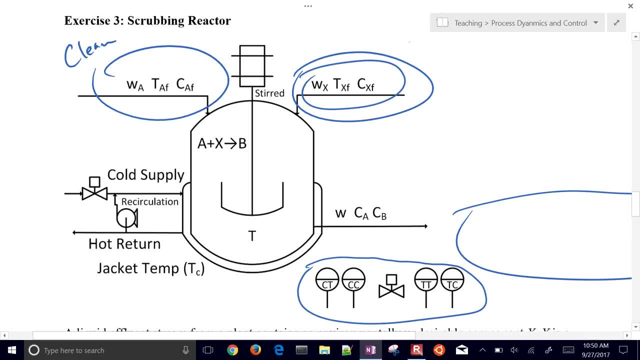 that this is going to be coming. we just need to treat this stream. okay. we need to clean. this is our dirty stream, with this component X in it that we want to get rid of, and this is our cleaning agent right there. so we might put, for example, a valve on this to be able to adjust it. so I'm just going to include. 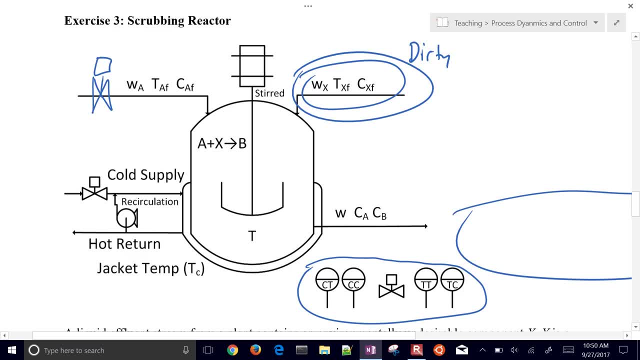 the valve right there and then I could have manual operation. for example, I get open or shut that as I see the concentration changing on this inlet line. okay, so I could put a concentration transmitter here. okay, but that you can see that it's not going to be able to get rid of and this is our cleaning agent right there, so we might put for. 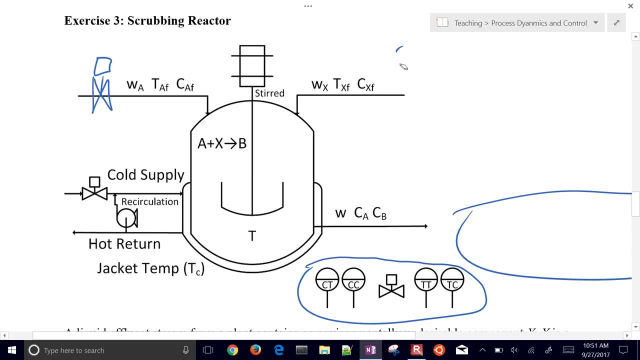 example, a valve on this to be able to get rid of- and this is our cleaning agent right there, so we might put for isn't really a thing that I'm trying to control. the thing that I'm trying to control is actually what's coming out of the reactor. so for a feedback controller. 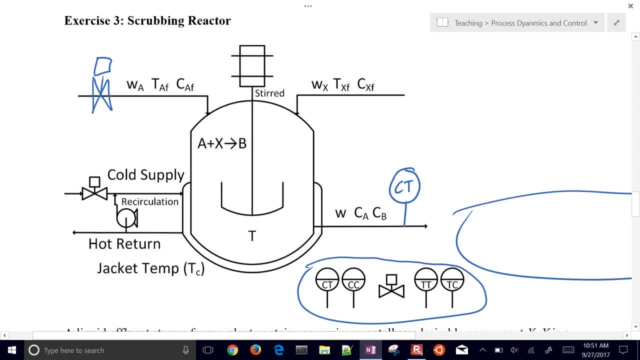 I'd want to put a concentration transmitter here and then that would feed into a concentration controller and then that concentration controller is going to send a signal to the valve to open or shut, to add either more or less a to be able to run the system, and then that would be able to run the system. 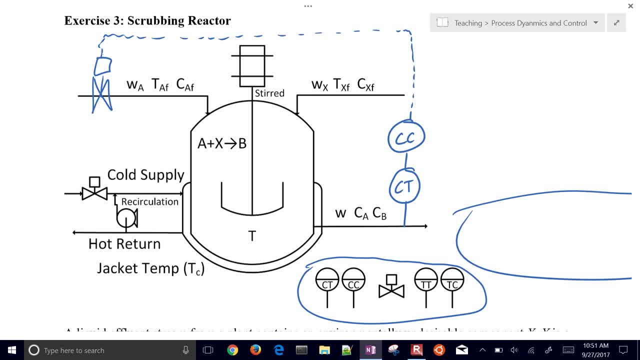 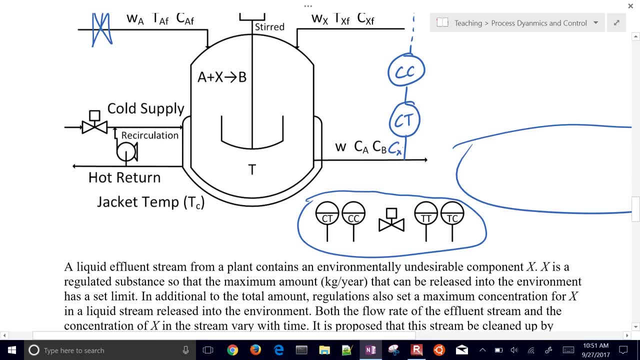 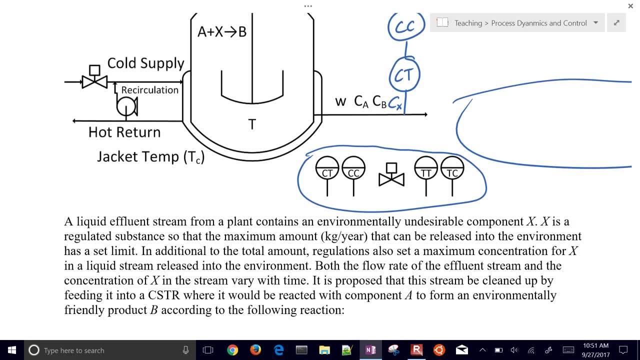 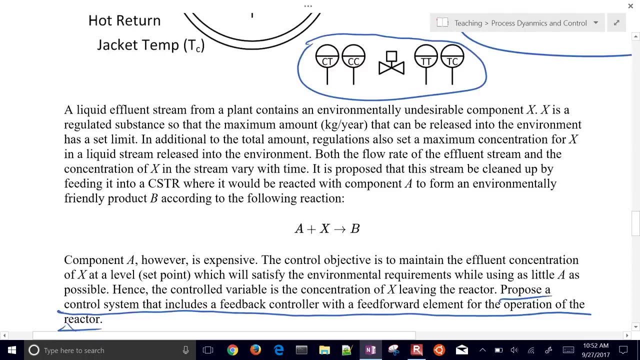 regulate the amount of X that's coming out of the reactor. okay, and I guess I should have added one other thing here, which would be concentration of X. that's the one that we're interested in, that's the one that we want to make sure we don't go above a certain amount on that, okay, okay. so there's our feedback. 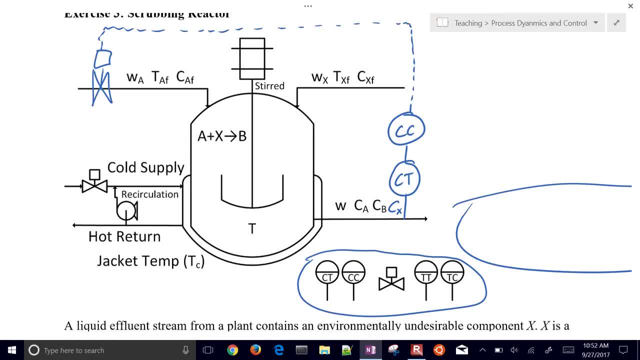 control system right here now we might want to add a feed forward element like: let's say, we want to add a feed forward element like: let's say, we want to add a feed forward element like: let's say: this concentration is significantly changing, for example. or let's say, our. 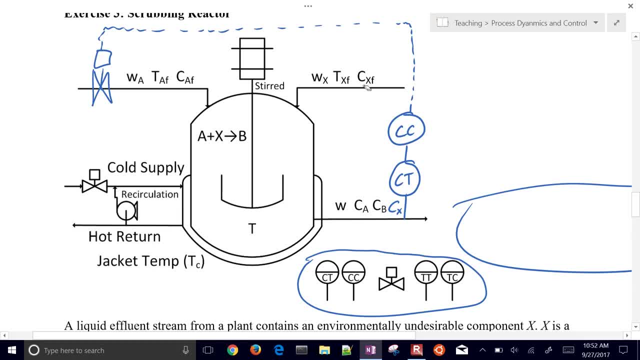 our kinetics, you know, depend on the temperature in the reactor. then I could add a feed forward element by adding a temperature transmitter here. okay, and that is, then I'm going to draw it on the other side, just so it can feed into the controller temperature transmitter and that information is going to feed into 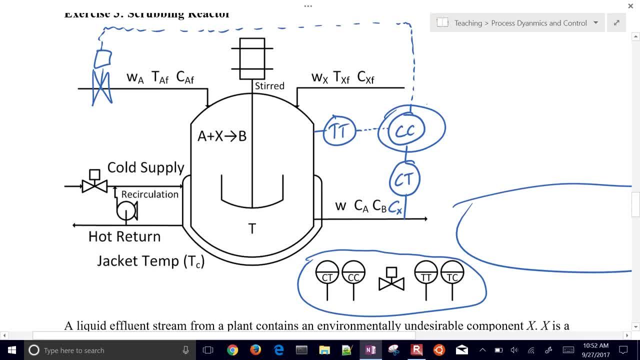 this concentration control system controller right here to is. it sees maybe if the temperature drops it will proactively add a little bit more a in order to maintain the outlet concentration that we desire. so feed forward tries to anticipate disturbances, measures them, like temperature in this case, and then proactively adjusts the. 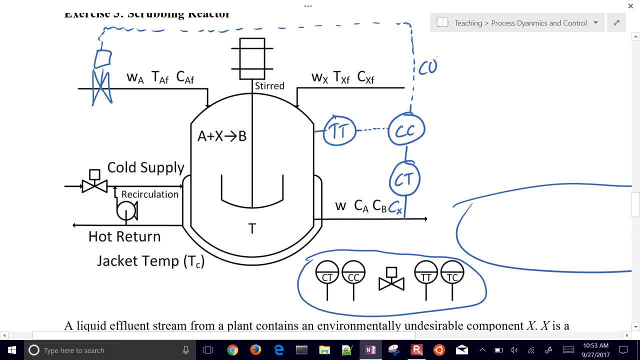 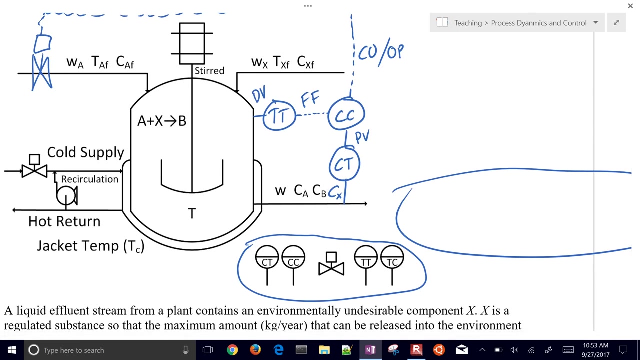 control output. okay, so this is going to be the controller output, or we also call this the OP. this concentration transmitter is going to be sending the PV process variable to the concentration controller and this is going to be our feed forward element, measuring the disturbance variable. so that is a feedback with feed forward. let's go draw a block diagram as well. 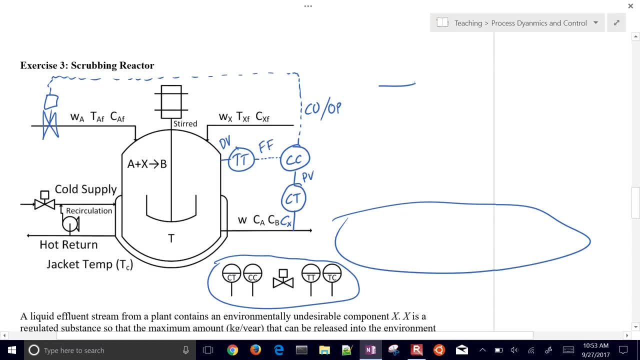 for the system just to show the flow of information. we have a setpoint and that's going to be for our concentration of x leaving the reactor. we're going to compare that. so i'll put a plus and a minus with our pv, our process variable. but we get our process variable from the sensor. 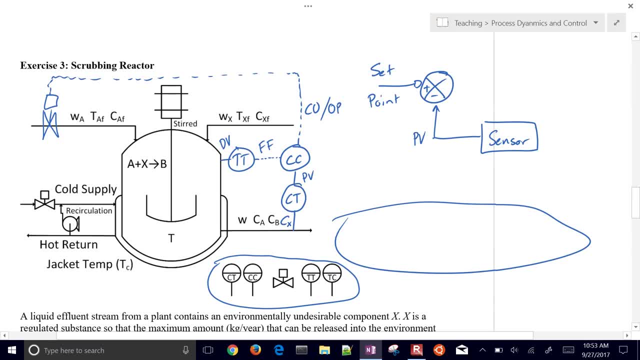 in this case it's going to be from the concentration transmitter, okay, and then i'm going to be sending this. this is going to be my error between my set point and my pv, and that's going to be sent to a pid controller, some sort of controller, and that. 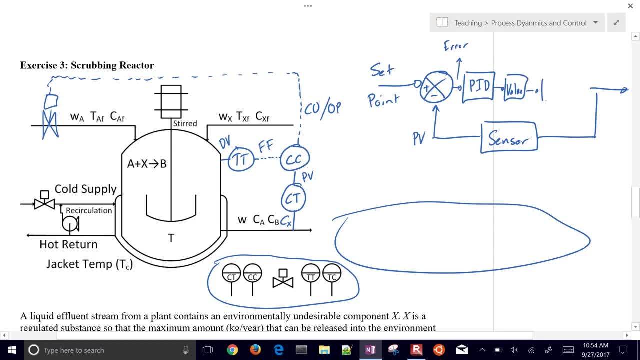 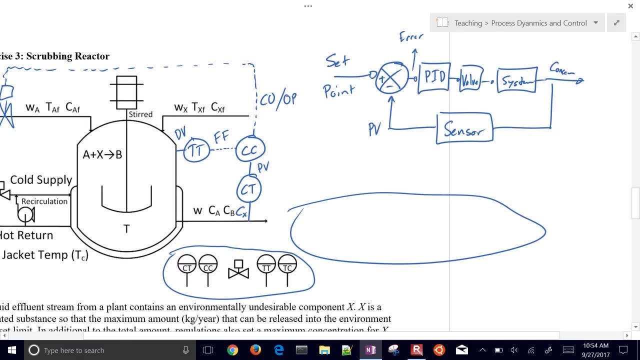 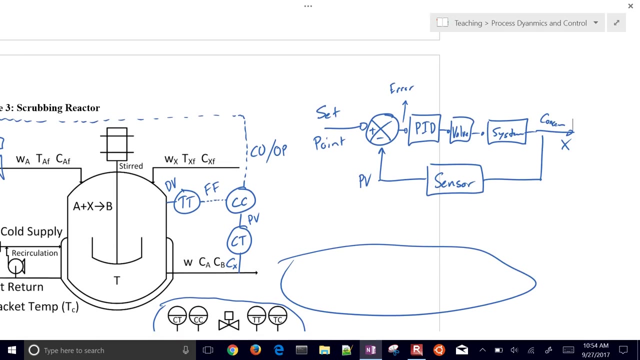 goes to a valve and then that affects my system, so that valve opening or shutting is then going to affect the outlet concentration and so this is going to be my concentration of x coming out. so this is a feedback control system and then if i added the disturbance- okay, in this case it was temperature- 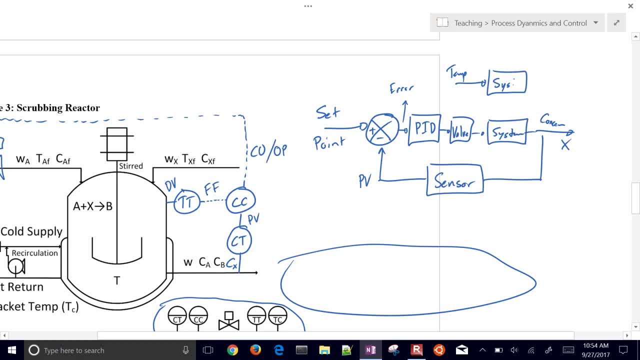 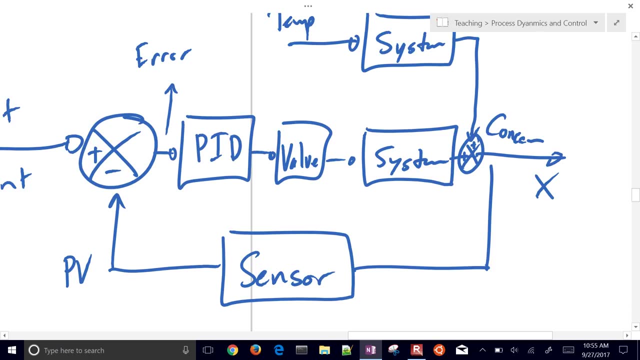 and this is a process model of my system- how temperature affects my outlet concentration. and then i would just add that in right here. let me just zoom in on that. i would typically put a plus here and a plus there, so i'm just adding the effect of how the valve affects. 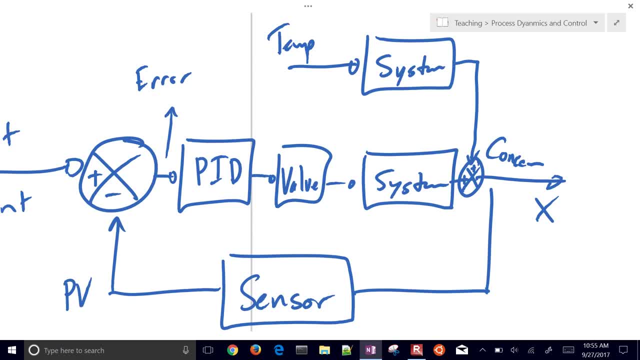 you know, opening or shutting, and then i'm going to be sending this to my pv, and then i'm going to be sending this to my pv, and then i'm going to be sending this to my pv and then i'm going to shutting. how that affects the concentration and also how the temperature affects. 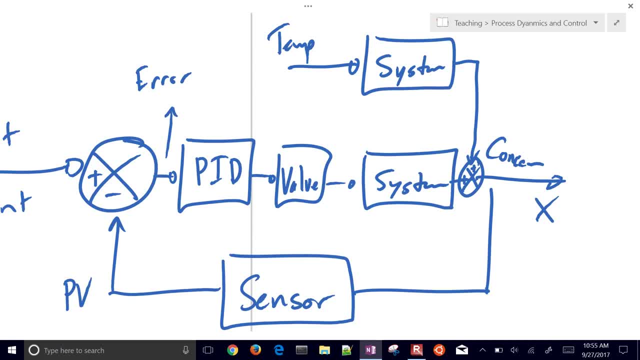 the concentration. now i can add a feed forward element to the controller by adding something like feed forward right here and then that would then add in right down here. i'll just put a plus and a plus there. you can't really see that- and i'll draw those boxes around these two again. 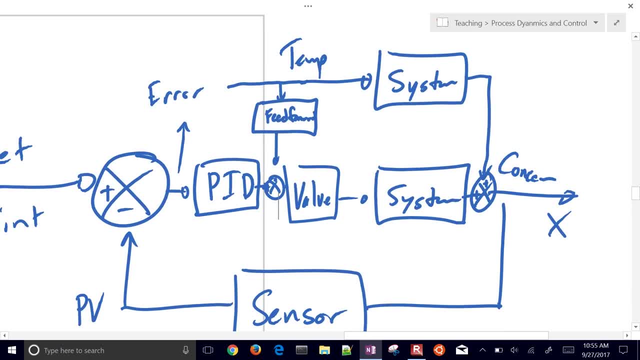 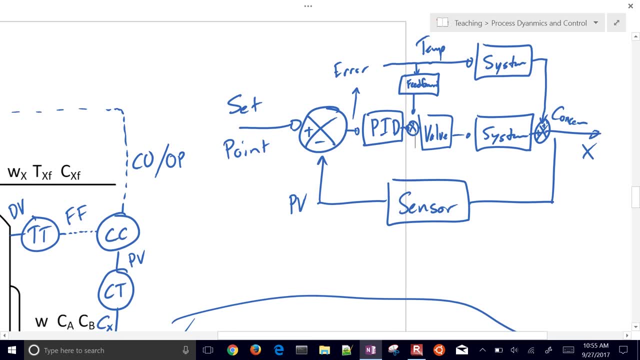 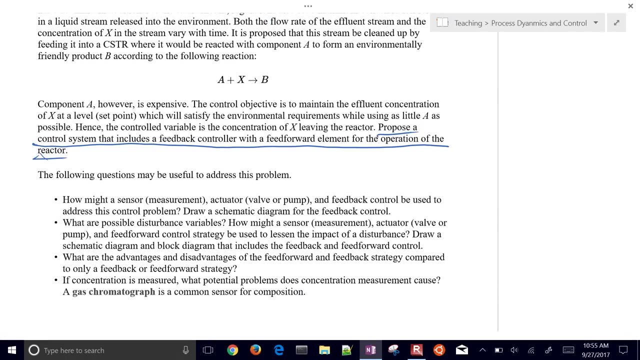 uh, so it's getting a little bit squished there, but i'm just adding in the feed forward element there to the pid output and it's included in the pid controller. okay, so there's a block diagram that shows the flow of information for this control system. okay, so there's our 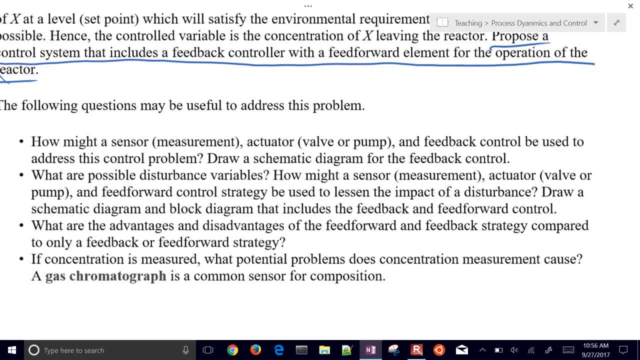 let's try to answer the remainder of these questions. how am i, a sensor actuator and feedback control be used to address this control problem? we drew the schematic diagram for the feedback controller and also the block diagram. what are the possible disturbance variables? We talked about temperature, but it could be changes in flow rate or other. 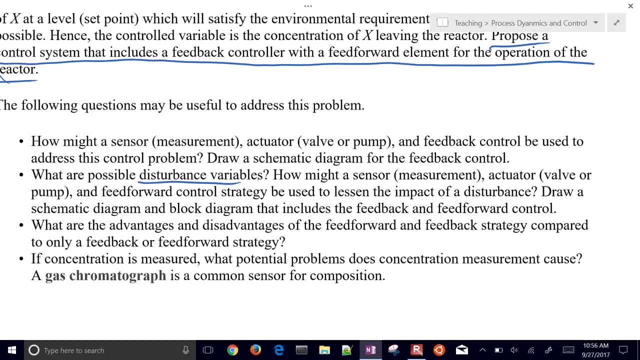 conditions that would affect the concentration coming out. And then we suggested one sensor to be used as a feed forward, which was measuring the temperature of our reactor. And okay, then we drew the block diagram and the schematic that shows the feedback and the feed forward control. So what are the advantages and disadvantages of the feed forward and feedback? 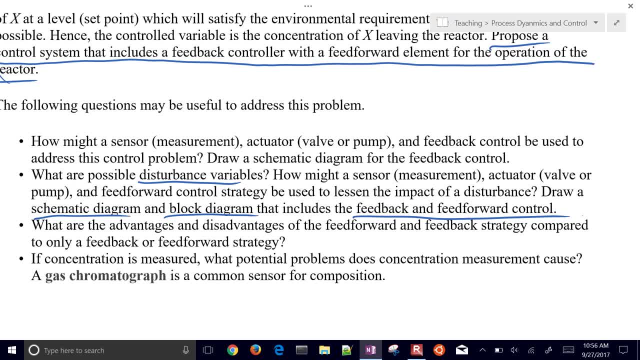 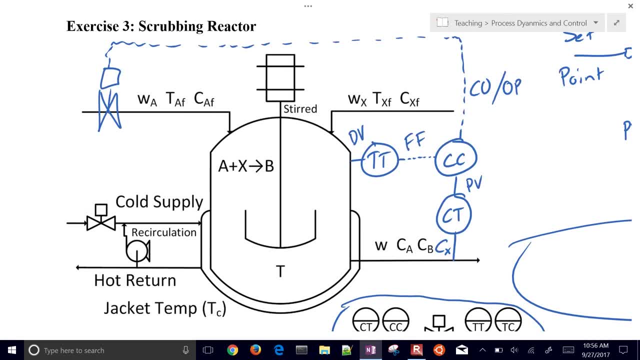 strategy compared to only a feedback or feed forward strategy. So if you come back here, one of the things to just review is, if you only measured, for example, the temperature in the reactor and try to adjust the valve to maintain an outlet concentration, you weren't. 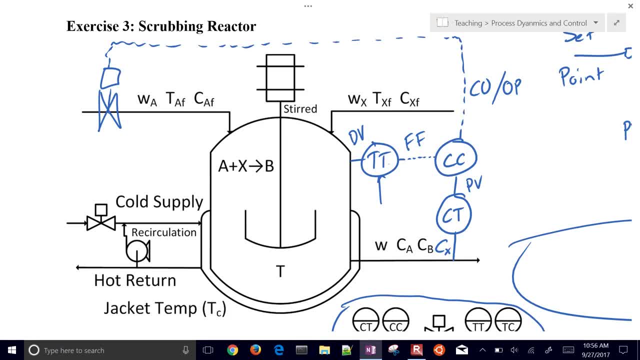 measuring the concentration coming out, you'd likely not meet your set point. So very rarely is a feed forward controller ever used without a feedback controller. So typically there's a feedback controller and then sometimes you add a feed forward element to that to help it improve its ability to reject disturbances that drive you away from the set. 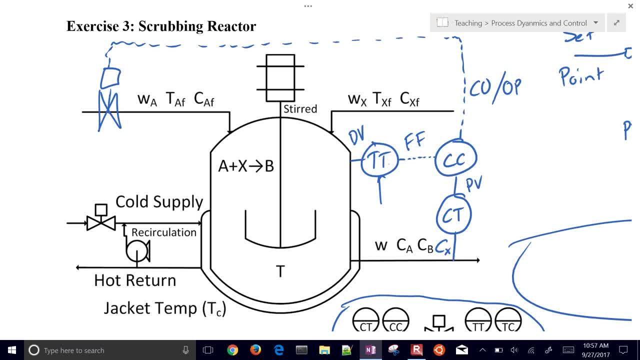 point. So I just say feedback plus feed forward is more common. There's very few cases of just feed forward only. Okay, so feedback versus feedback plus feed forward. Feed forward is going to help you to then reject disturbances that are caused by a change in temperature And so often, your control. 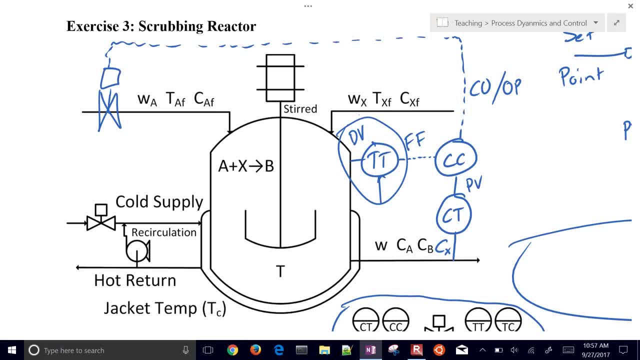 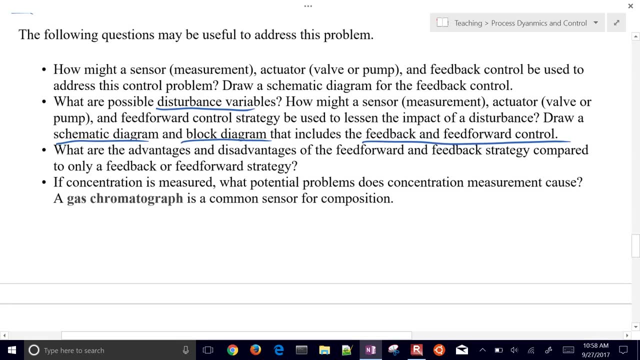 can improve. So what people often do is they implement the feedback first and then, if there are disturbances that are affecting the process repeatedly and you can measure that disturbance, then you can add a feed forward element. Okay, so also concentration is measured. What potential? 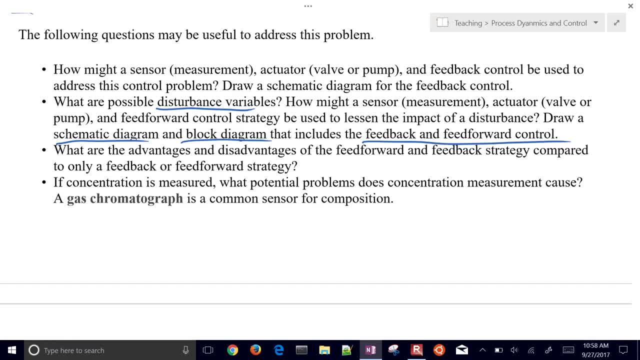 problems does concentration measurement cause? So in this case the signal was very low, it was very light. So we did a measure of 10 seconds and it showed that it was very low. We tried to measure the temperature at 30 decibels per second, So when that is, it should be about 30 decibels per second, And then 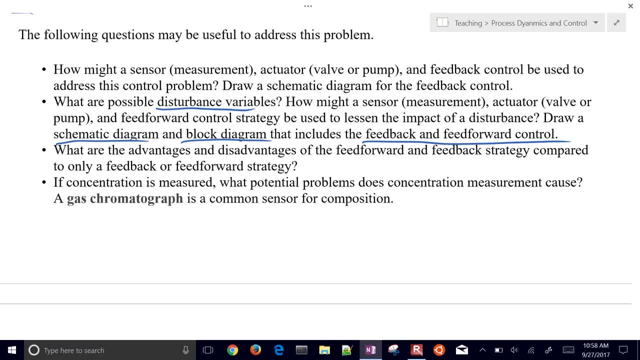 we measured it with the heat sink, and that's what we did. It showed that it was very low, So that was good. Then we measured the temperature at 30 degree Celsius. so at 30 degrees it was probably around 60 degrees Celsius, you know, but it was very low. So we did a little. 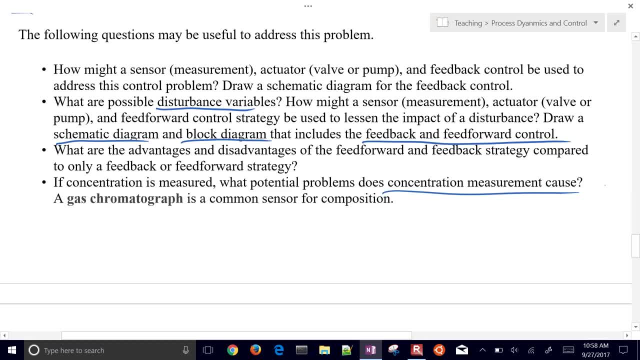 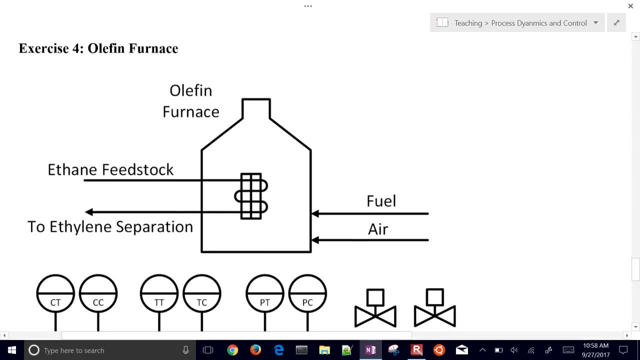 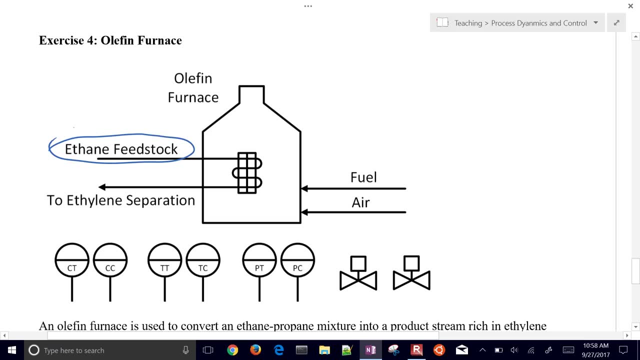 deeper measurement. Okay, Yeah, know the measurement technology that you're using and what effect that's going to have on your control system. okay, let's go on to the final example here. this is going to be an olefin furnace. now you have ethane feedstock right here and then use steam reforming to convert it to ethylene. 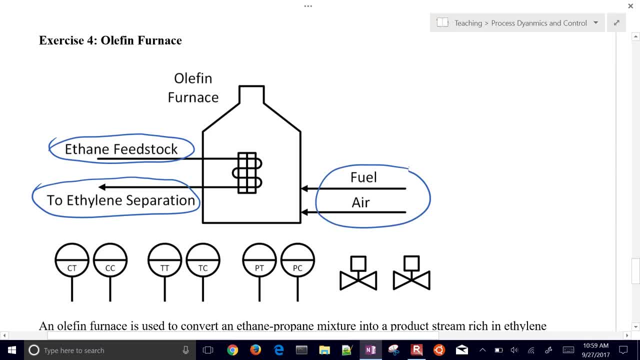 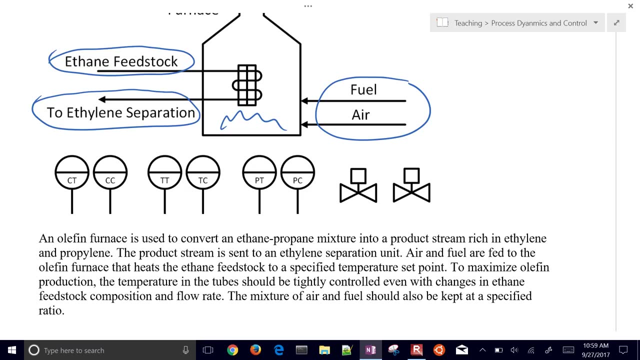 and you need to maintain this at a certain temperature. so you add fuel and air that then burn in here and heat these tubes. okay, and and you're trying to, um you know, convert this ethane propane mixture into a product stream rich in ethylene and propylene and the product stream 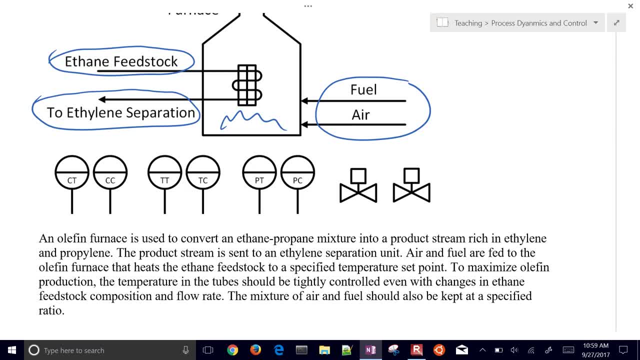 is then sent to an ethylene separation unit, where they have these, you know, big distillation columns that are operate, uh, very cold to separate these two components. but we have the air and in this furnace we have the air and the fuel are fed to the olefin furnace that heats the ethane feedstock to a specified temperature set point. 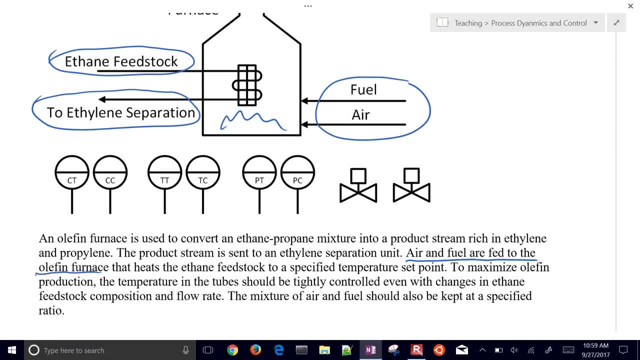 and then to maximize all of the production. the temperature in the tubes should be tightly controlled, even with changes in ethane feedstock composition and flow rate. okay, so this flow right here might be changing, or the composition might be changing as well, and we want to design a control system that can adjust the fuel and air to be able to maintain a 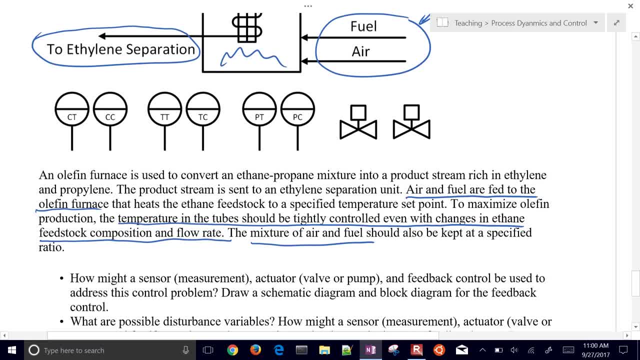 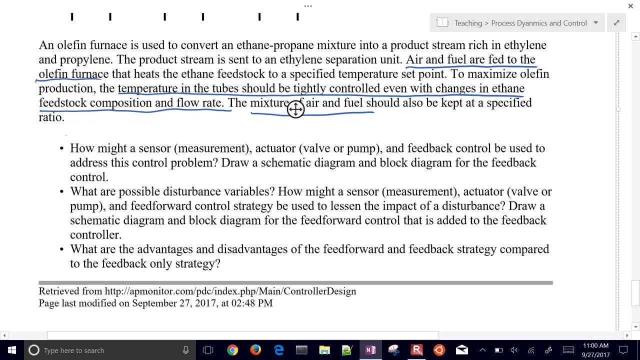 temperature. we also want to make sure that the mixture of fuel and air should be kept at a specified ratio, so we might have something like a ratio controller there. so if i'm adding this much fuel, i need- no, i need- to add at least this much air to the system. okay, so how? how might a 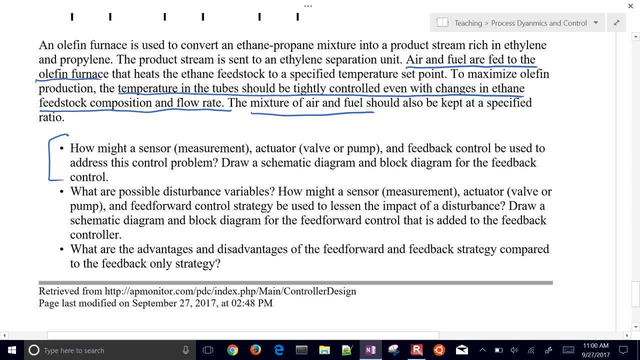 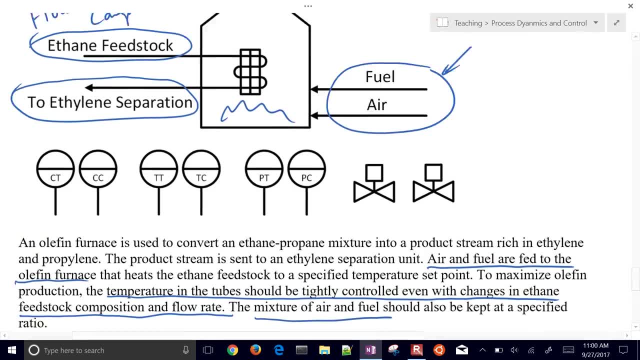 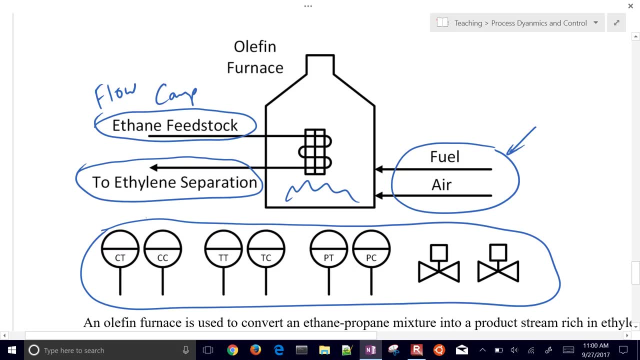 sensor, actuator and controller be used to address this control problem. well, first of all, draw schematic diagram and block diagram for the feedback control system. we have all this. you know, maybe we have these, uh, these sensors and actuators right here, okay, so let's go ahead and think about how we might do that. so you know, we're not really trying. 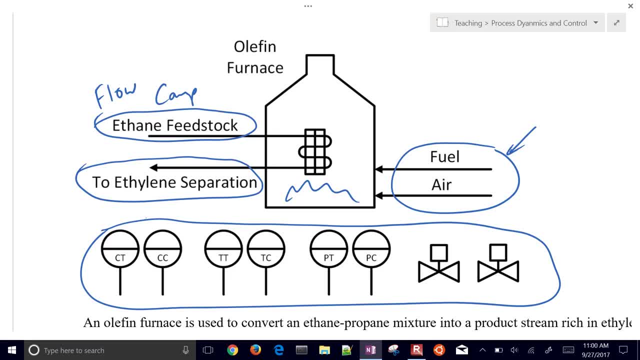 to measure, control, composition, but it's really the temperature inside this system that we want to try to measure and control. so i'm going to add one of these temperature transmitters. so i'm going to measure the temperature transmission sensor and control system. so i'm going to add one of those. 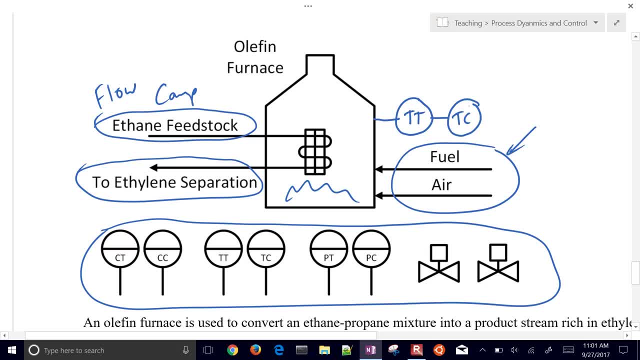 and i'm going to move the signal to this temperature controller here that i'll be using, that i'm going to be trying to control, and then i might have a temperature controller right here that would adjust then the flow of fuel to this- uh, to this furnace. so here's a feedback control. 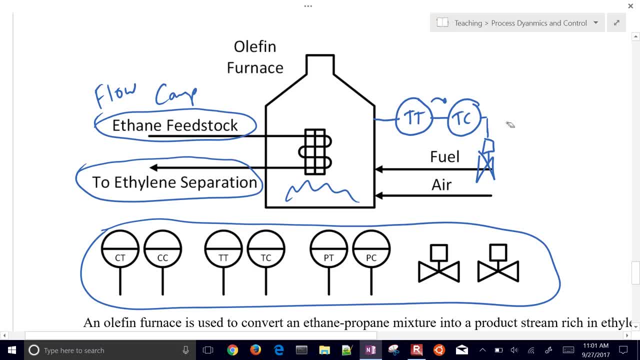 system. the temperature transmitter sends measures of temperature, sends a signal to the temperature based on if it's too high or too low, and then we might have a ratio controller or something like that that's tied, um, you know, between these two just to maintain a certain airflow, um and that. 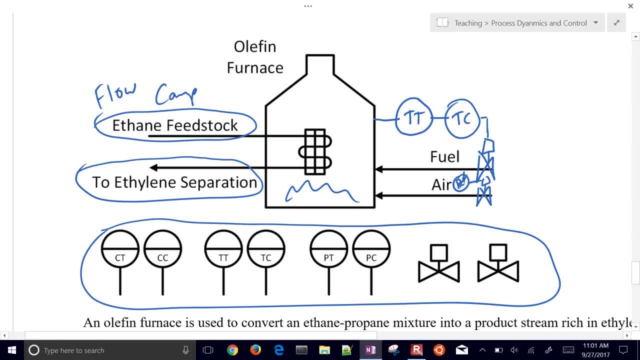 would be like a ratio controller that would then come into the valve. okay, to maintain a certain ratio of fuel to air. okay, but let's just uh, let's just focus on this uh feedback control system here for the fuel. we'll just assume that the air is able to be maintained in ratio to the fuel, okay. 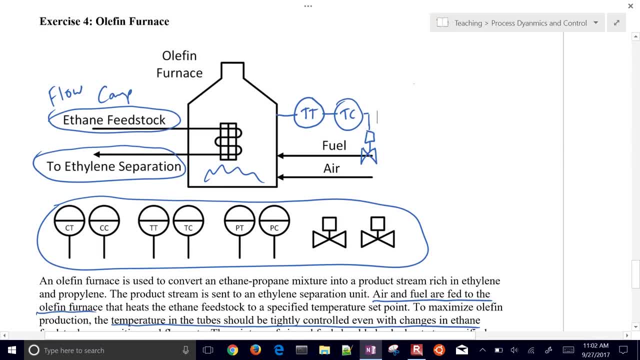 and let's draw our block diagram. we have a set point which is going to be our temperature in our furnace, and then i'm going to draw this a little bit bigger. here i'll do a plus and a minus and this is going to be our process variable. we're going to compare those. 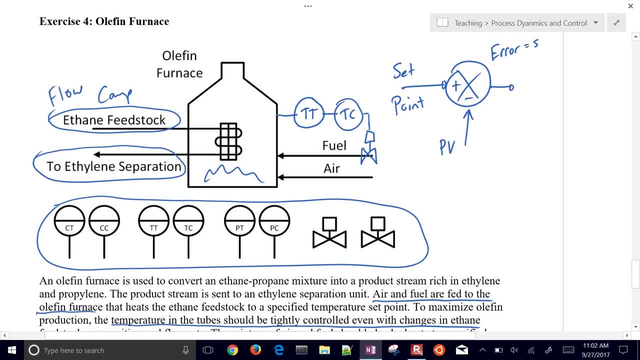 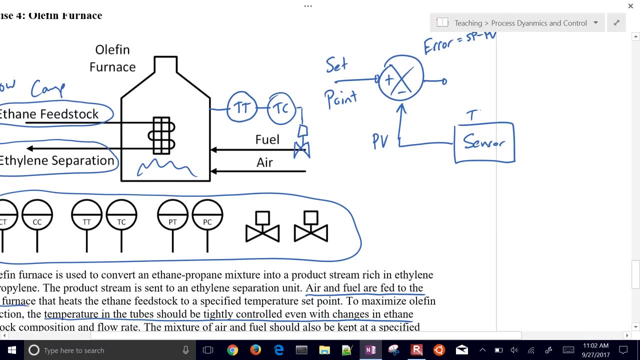 two and there's going to be an error between them. so air is going to be set point minus pv and that that process variable, the measured process variable, comes from our sensor. in this case it's going to be our temperature transmitter, that's going to be our sensor, and then that's going to 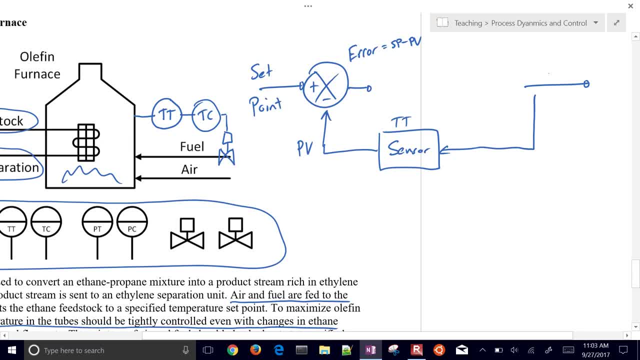 then be taken from the. the temperature of our process, okay, that we're trying to maintain. this air is going to be sent to something like a pid controller, which then manipulates a valve and the valve affects the process. so this is the whole furnace, the furnace process and it relates it. this is a model of the. the thing coming into this is the. 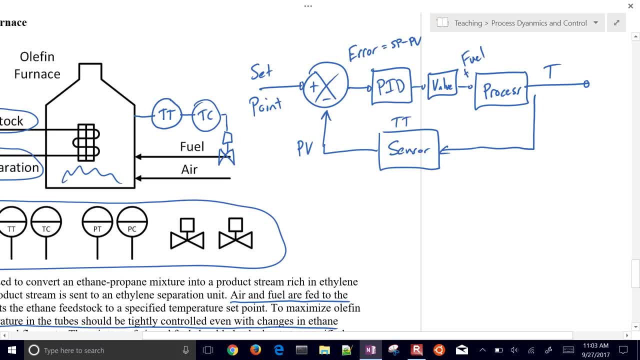 fuel flow flow and the thing coming out is our new temperature. so it's just a compact way to represent, if i have an increase in fuel flow, that this is how much increase i'm going to have in my corresponding temperature. so it's a block that relates input to the output. okay, and then, uh, you know, let's just 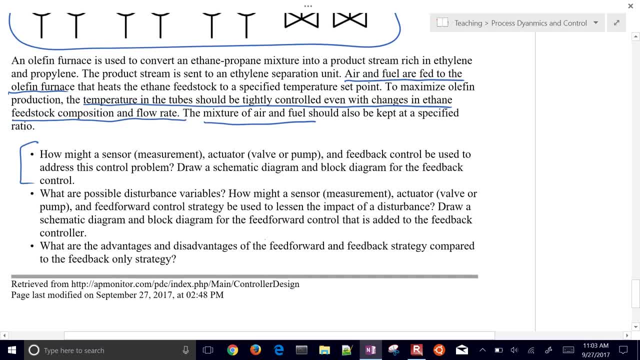 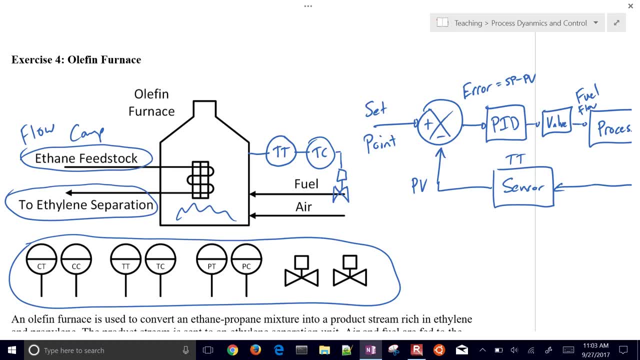 think about a a feed forward strategy as well. uh, you know what could be affecting me? um, one of the things that's going to affect me when i'm building the process is each of these plans. of the things that we saw here was: uh, you know, the ethane feedstock flow or composition could change. 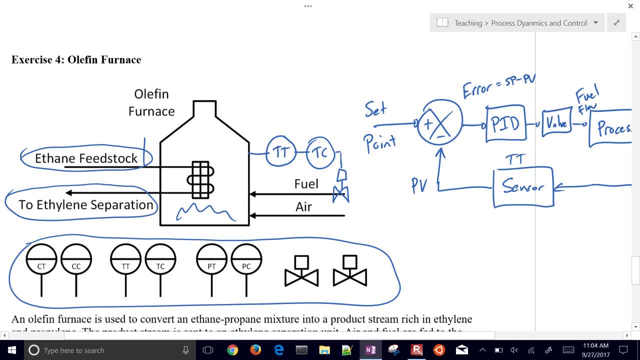 so we could try to analyze this, uh, this feedstock, like a concentration transmitter, or let's say we did have a flow transmitter as well. we didn't have that on our list, but you know, we could even have like a pressure transmitter. so either of these would work, we could even have. 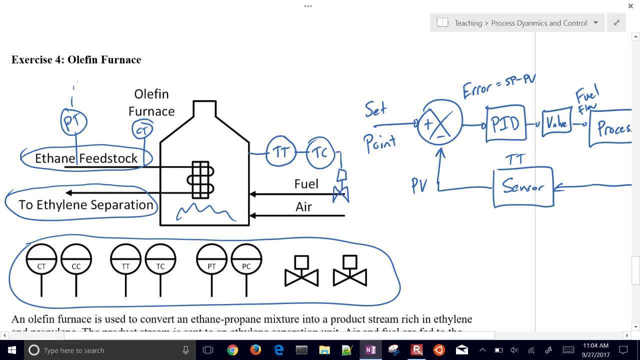 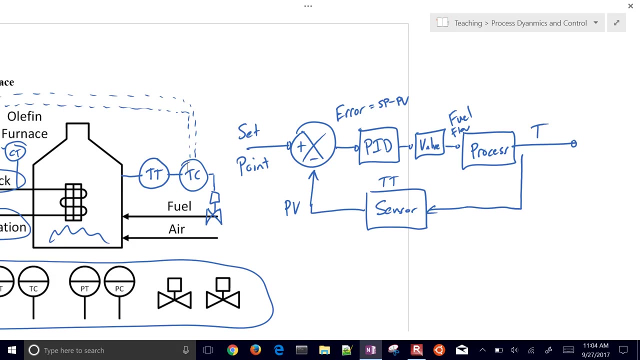 both of these. we could have concentration and pressure that then feed into the temperature controller and proactively adjust the output of the temperature controller based on disturbances that we see from the feedstock, from some other part that's going to cause a disturbance to our system. and so if i have those uh feed forward controllers, i have a couple disturbances. 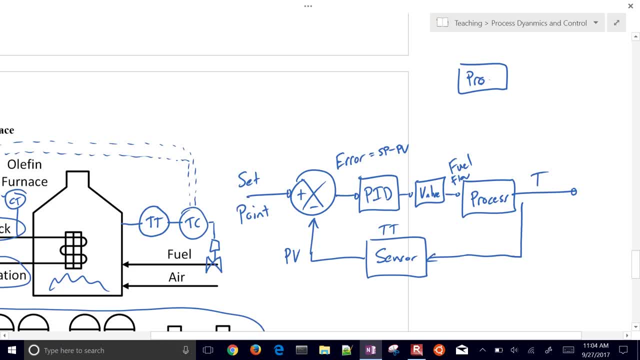 okay, so this is my process model of how the uh, this is how the temperature or the, the inlet composition, is going to affect temperature, for example. so this would be a composition of feed, okay, and then i'm going to just add this down here. actually, let me do this. i'll put some plus signs here. 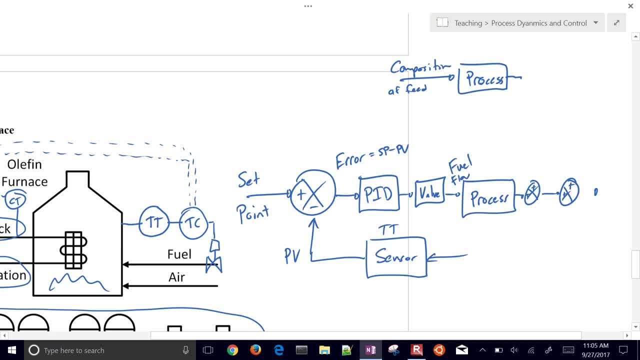 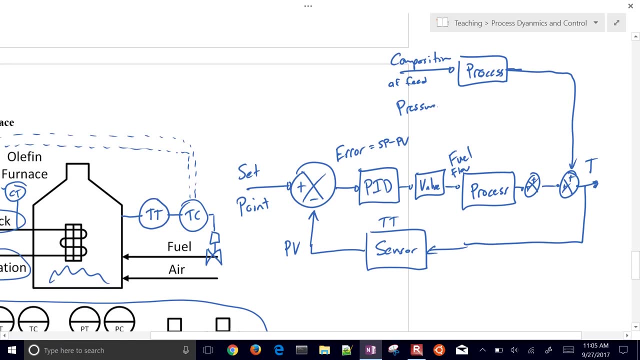 and then i'm also going to add some more plus signs here, because i have another one coming in as well. okay, so there's one and that's going to be my temperature being fed back, and then i also have my pressure- that's going to affect my flow- coming in for my ethane feedstock and that's also going to 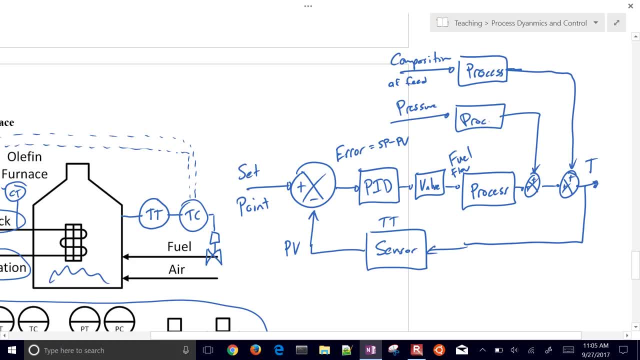 affect the temperature in the reactor. so these are all process models. they're different process models. it's how the pressure affects the temperature, it's how the composition affects the temperature, and then this bottom one is how the fuel flow affects the temperature. we're just going to add: 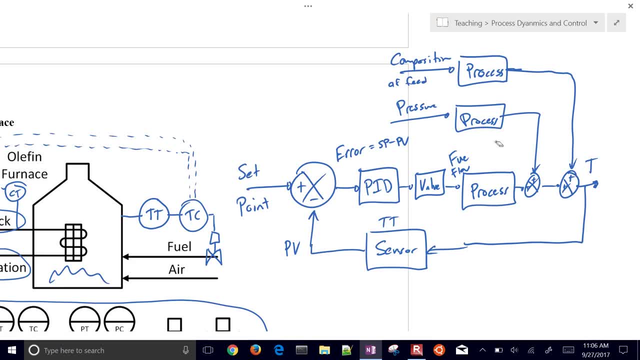 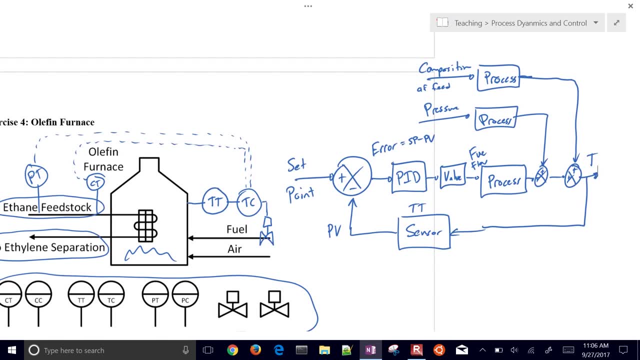 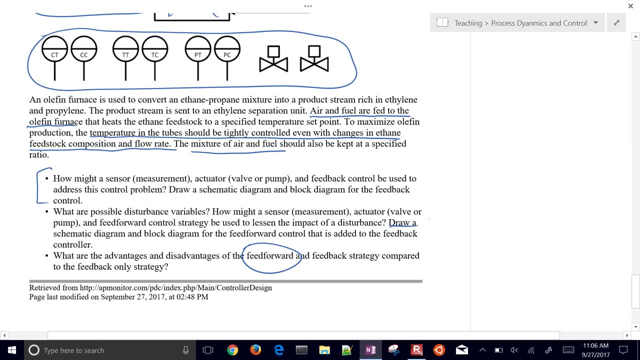 all of those effects together if we can assume linear models, and those are additives. so that's part of the reason why we use linear models in this course. but there's our block diagram right there. okay, so let's just see if we had answered all the questions. so we drew our schematic diagram. 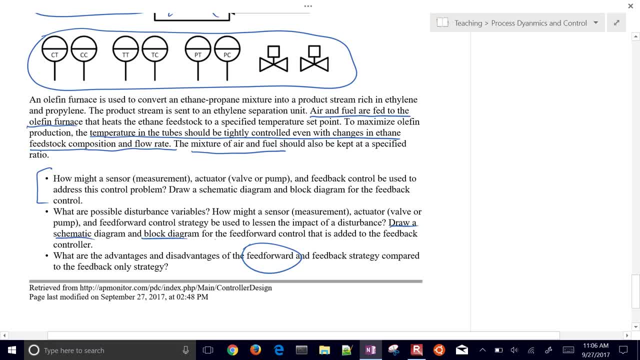 block diagram for the feed forward control that's added to the feedback controller and then just talk some of the benefits of adding the feed forward to that.